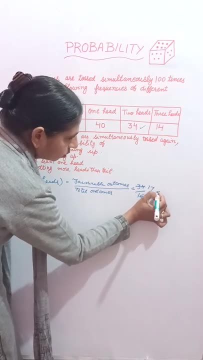 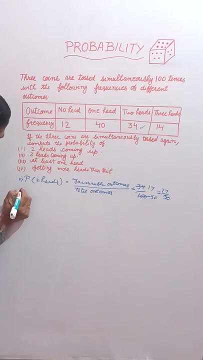 Cycling. When two heads are invested in one stock, it will show probability of three heads. So probability of one stock is any area your stock is listed. This is so critical If your stock, if you are making ten 2008,, 1000 home videos, sector scale, isiation, sugar for segurist. 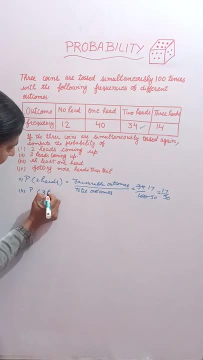 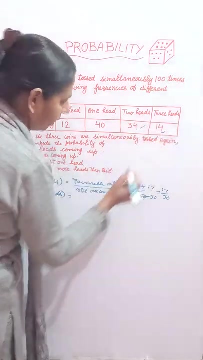 for the stock is Below 10 million. if your stock, if you so far there must be six, eight private companies, you can get up to 375, không h in Suribat From the first semester of a school incus per of three heads here favorable outcomes, three heads. so this is 14, 14 and total. 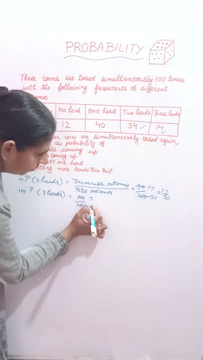 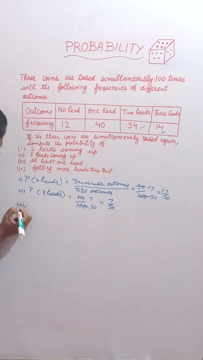 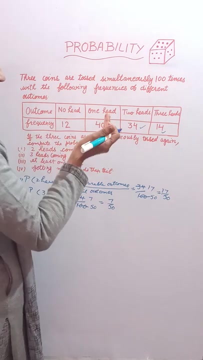 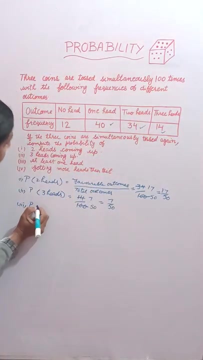 number of outcomes are hundred, so this is equal to 7 by 50. so this at least one head comes a come a head on a tree. second, a or a tree that also so comes a come a kind on. this is a dummy, who's at the right. so probability of at least one. 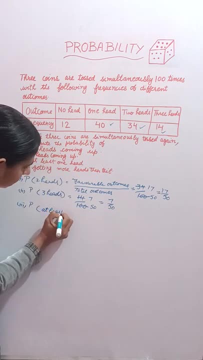 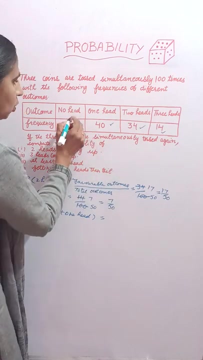 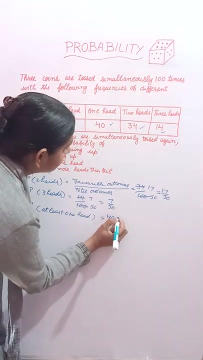 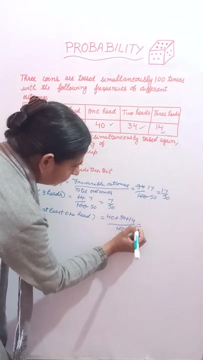 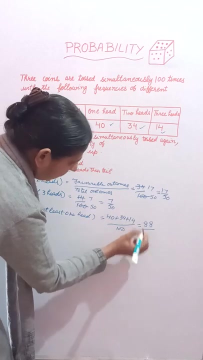 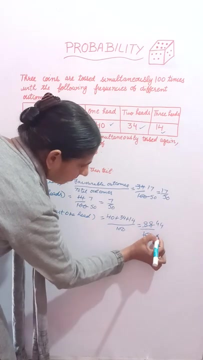 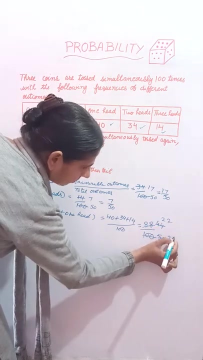 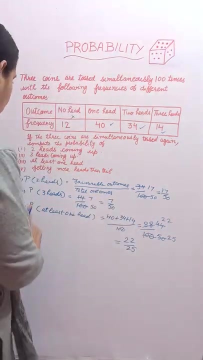 head here you will take favorable outcomes. no one we will not take because we have to take at least one right. so 40 plus 34 plus 14 over 100, 88 by 100. so we can do contain. so this is equal to 22 by 25 right now. probability of getting more heads than. 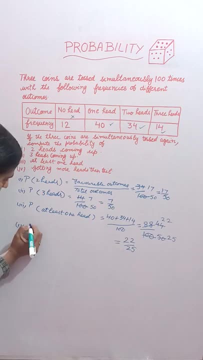 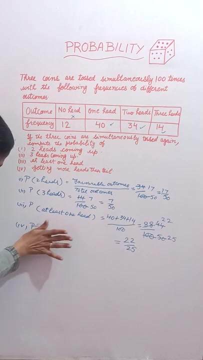 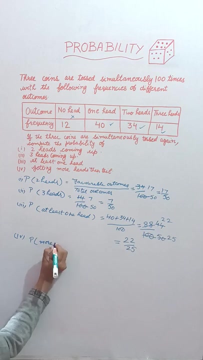 a probability of head much more heds than bid. so its equal to more head than a. that means so if it goes empiezais e r plus 1 than then, then you know that means on three heads less than one on. so your head value is 35.3 is equal to two. this 0.。